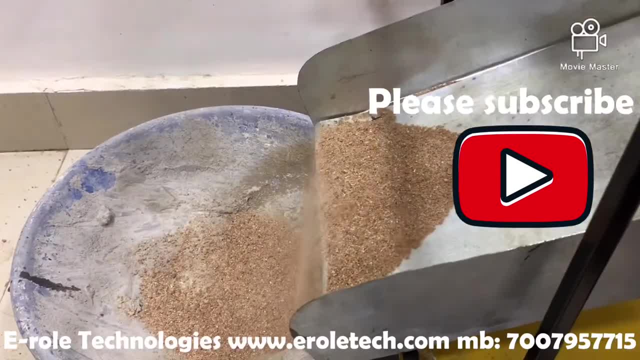 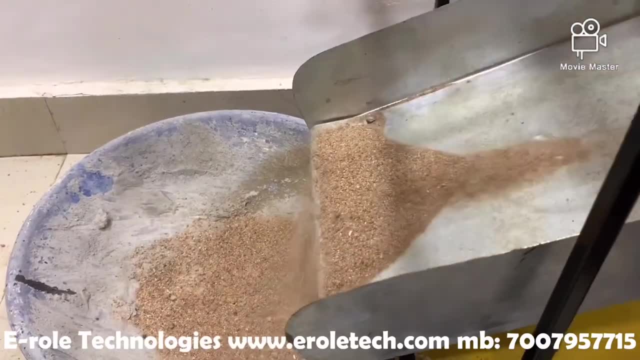 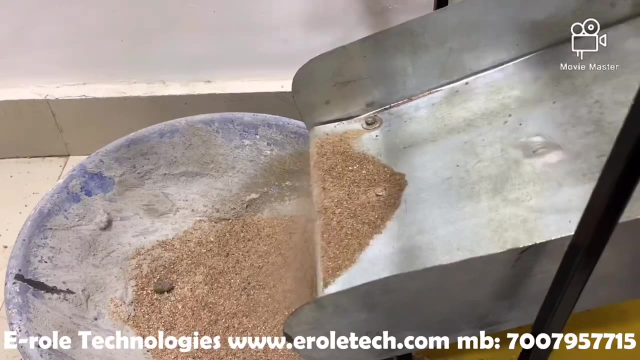 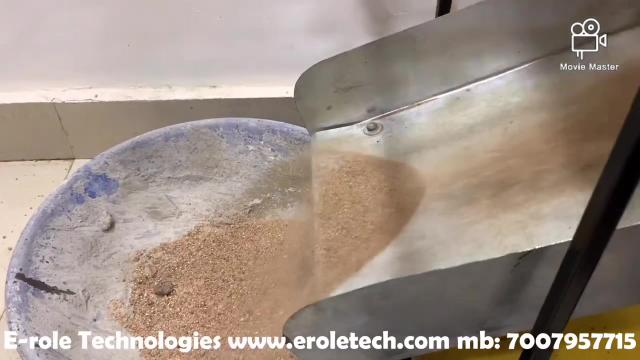 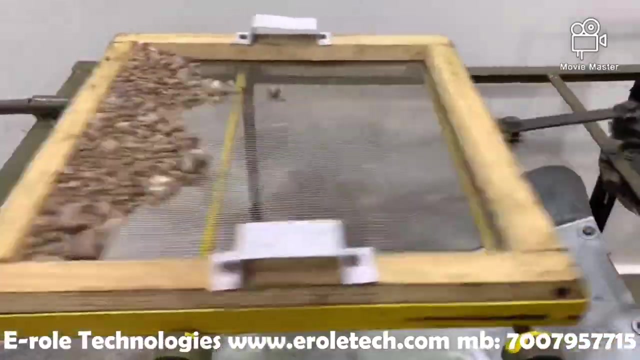 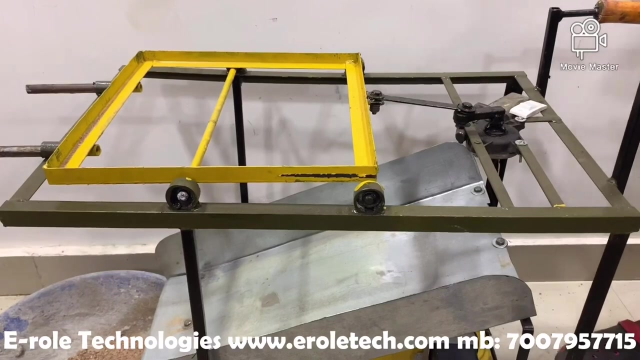 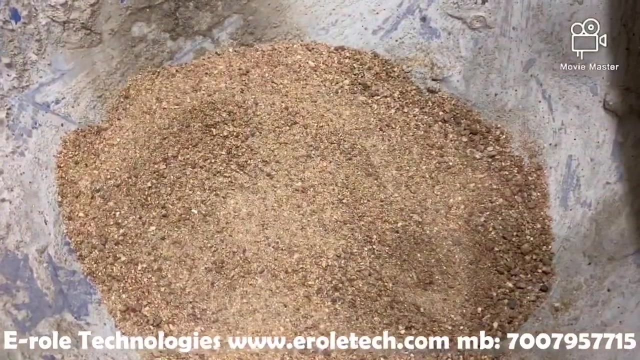 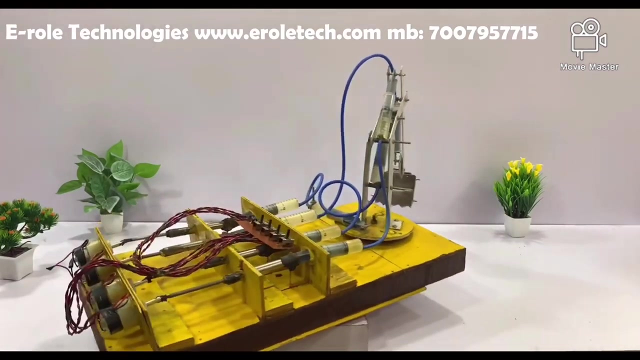 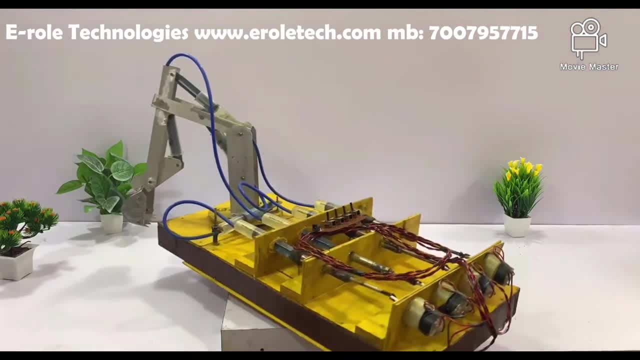 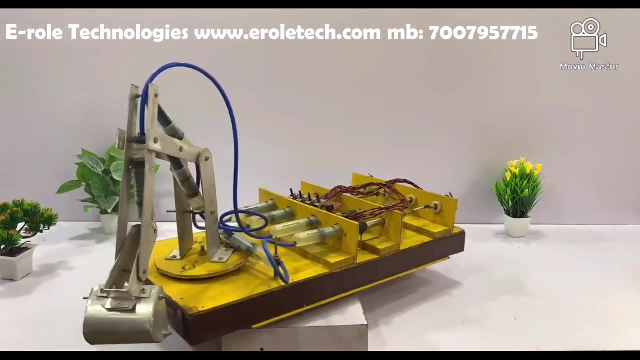 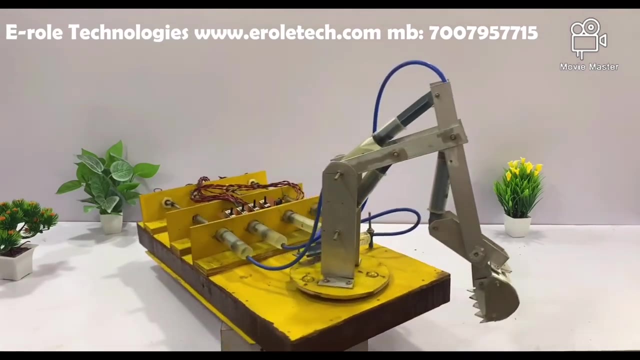 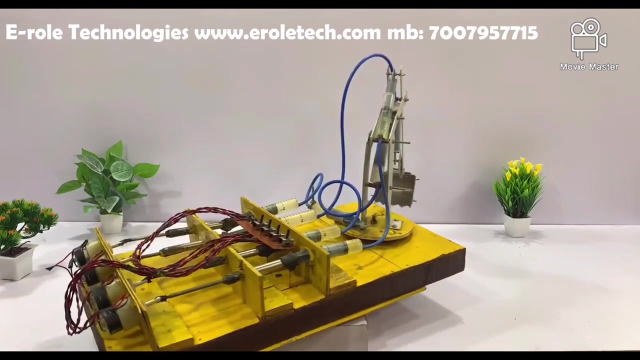 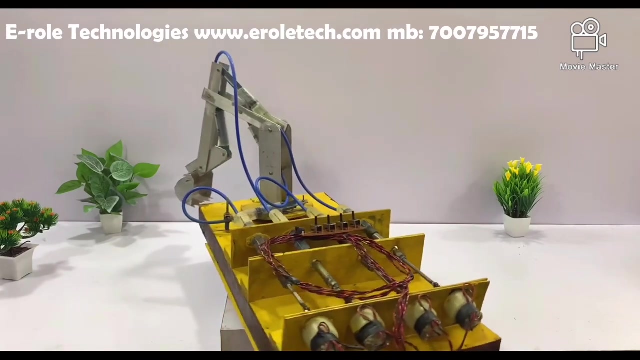 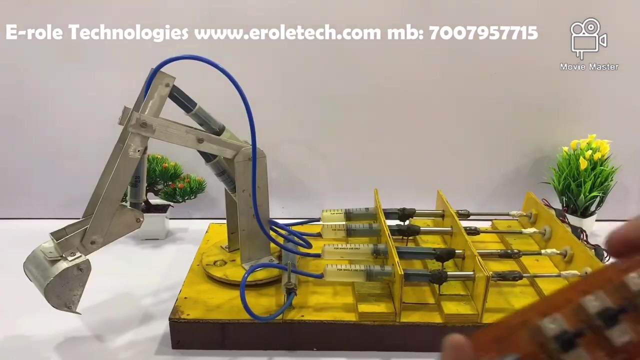 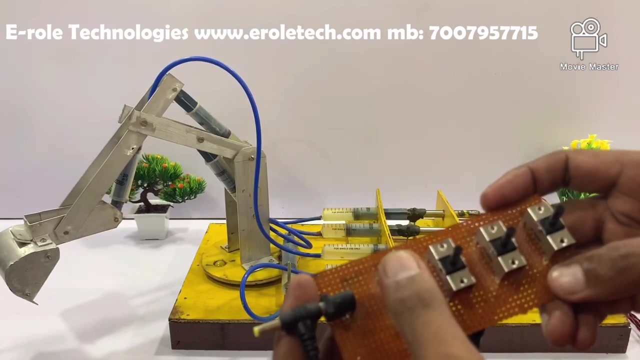 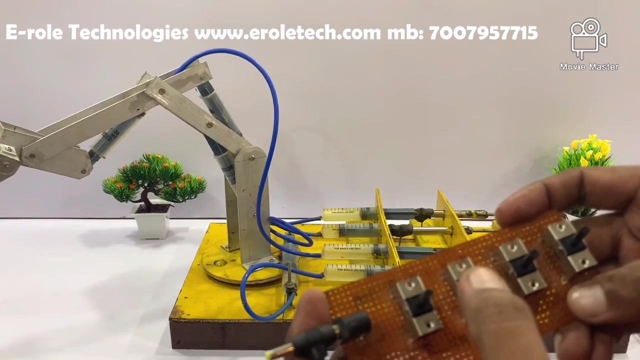 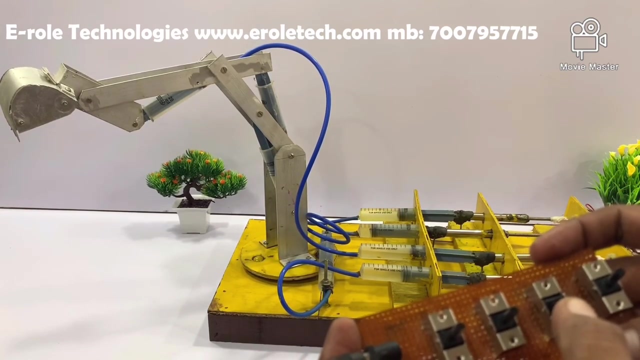 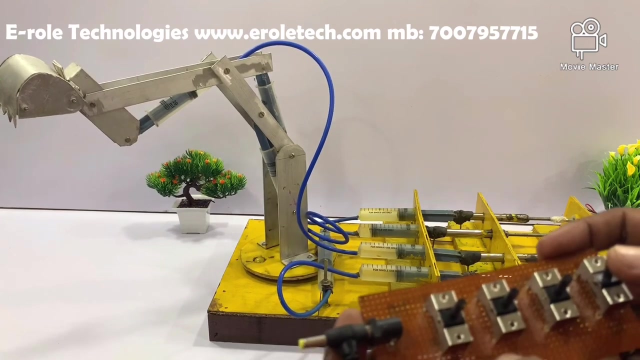 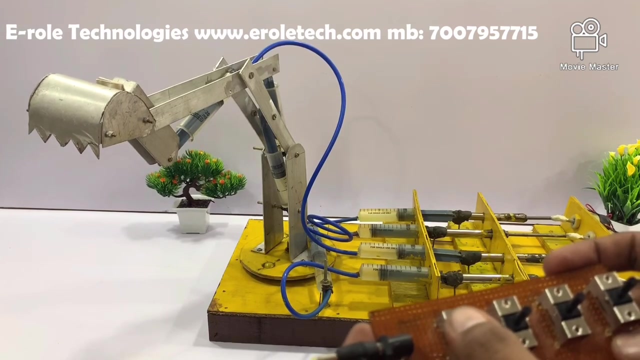 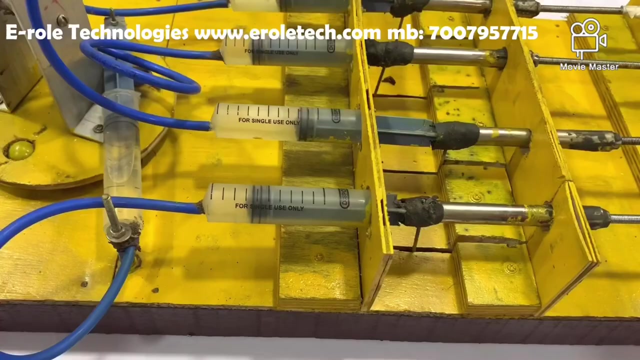 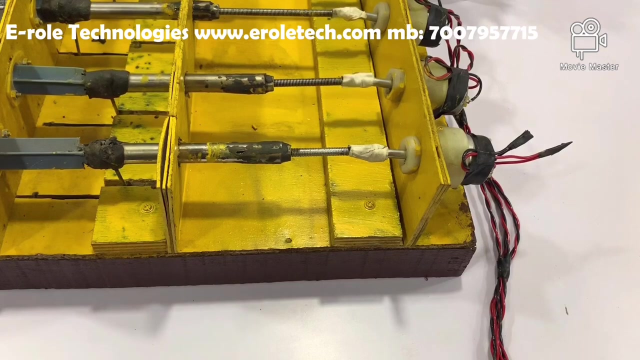 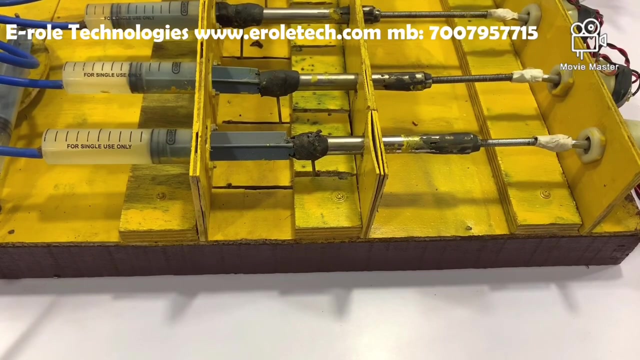 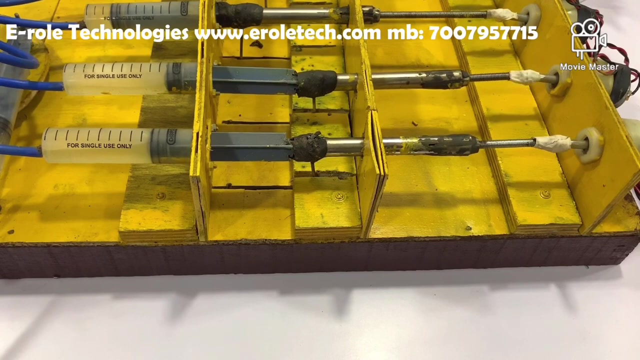 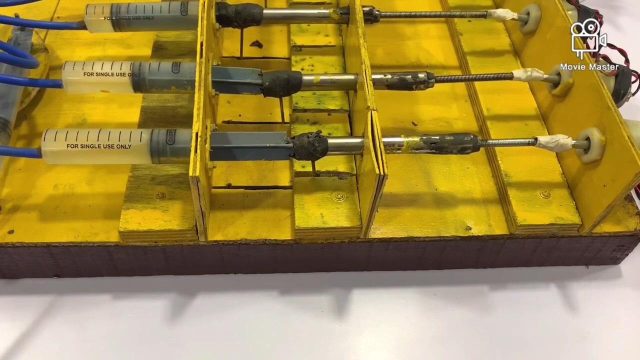 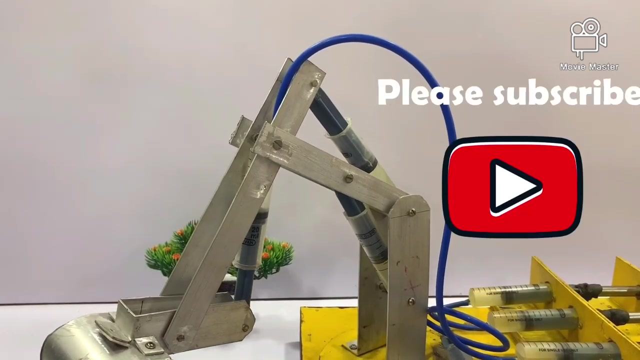 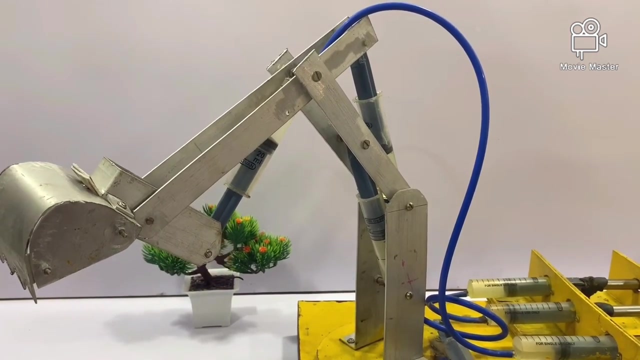 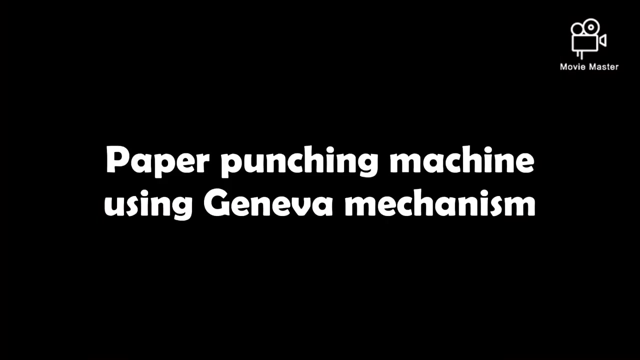 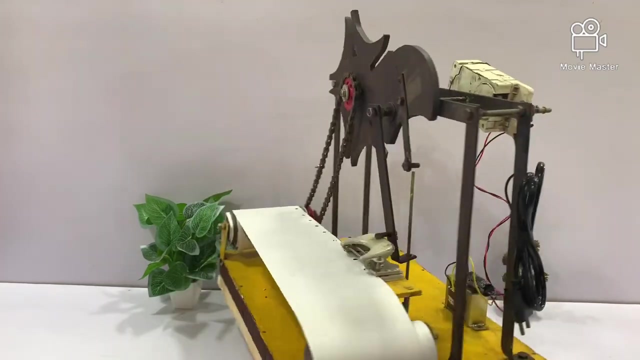 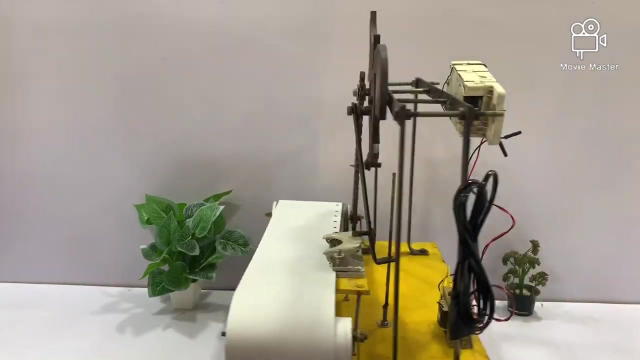 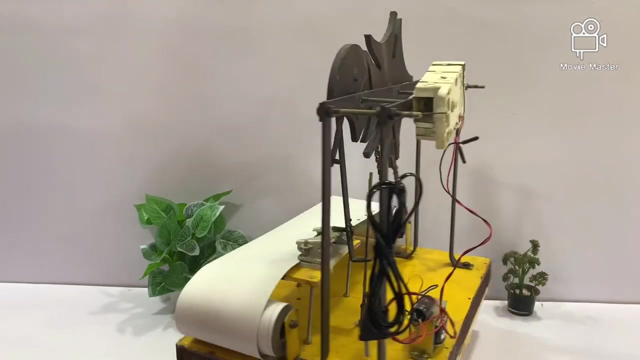 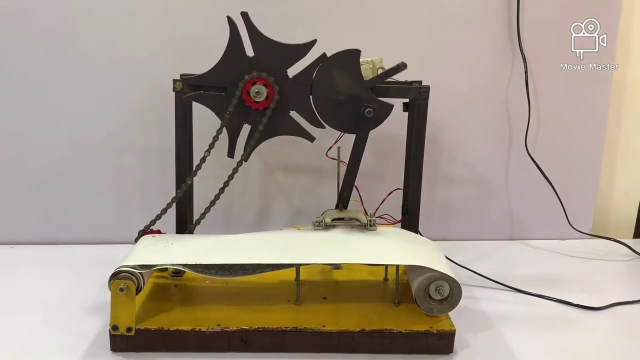 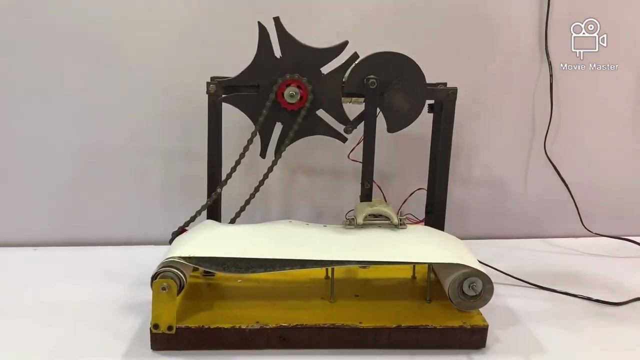 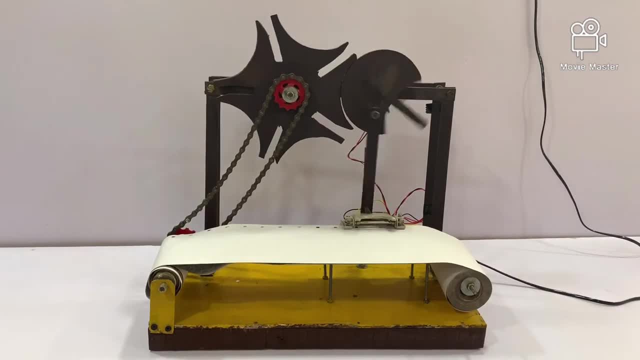 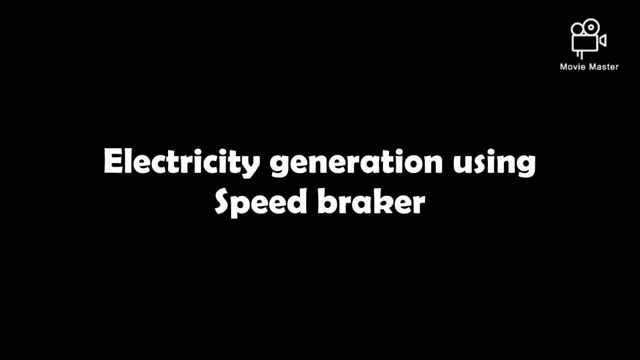 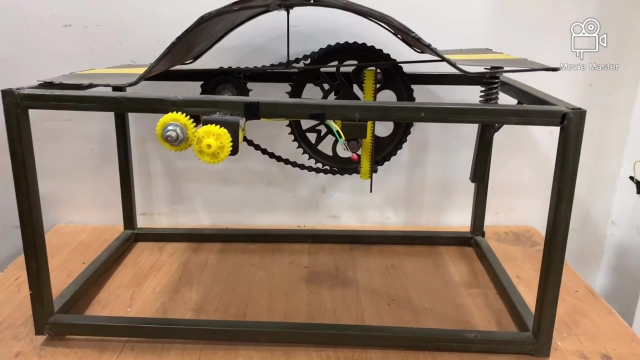 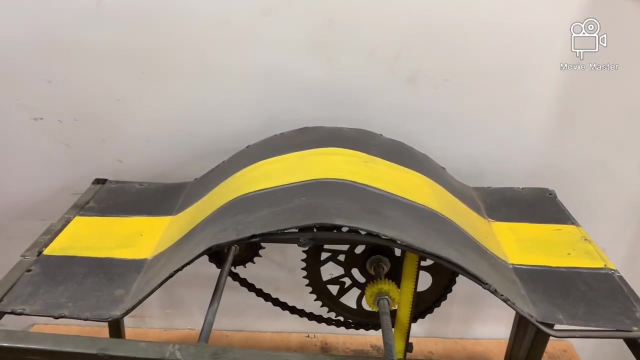 Step by step. The clock is ticking, But there's no time for regrets. I've been flying from town to town, From London to Taiwan. I've been all around the globe Trying to protect your soul. We are heroes tonight. We will fly above the sky. We are heroes tonight. 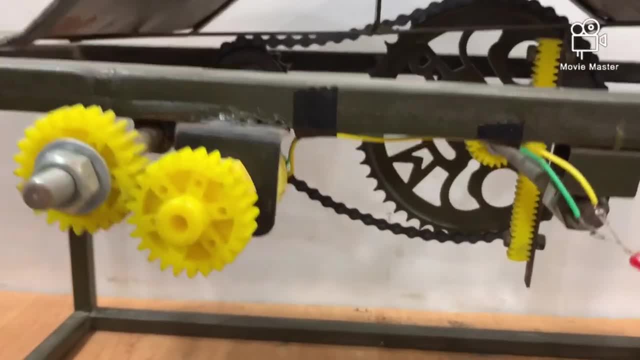 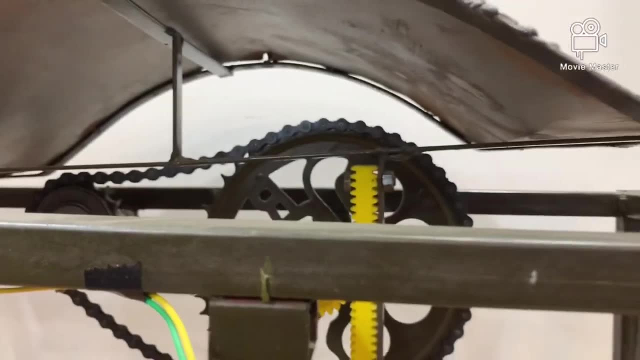 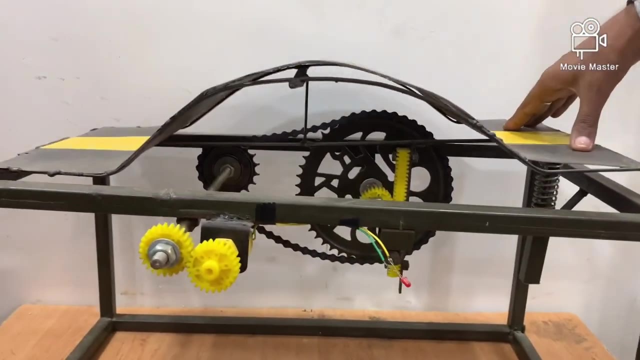 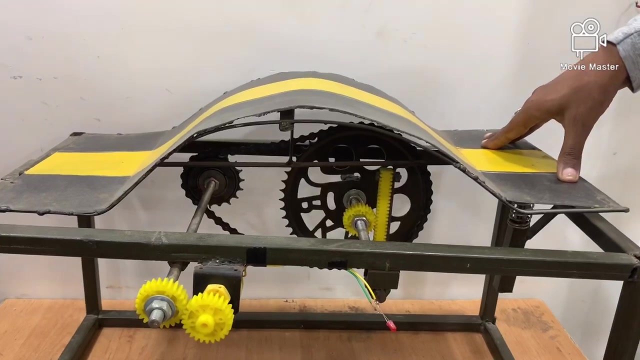 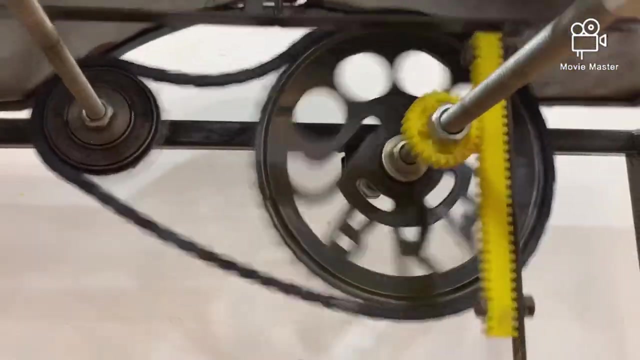 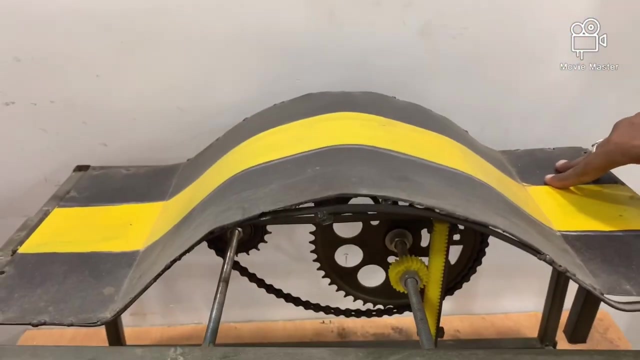 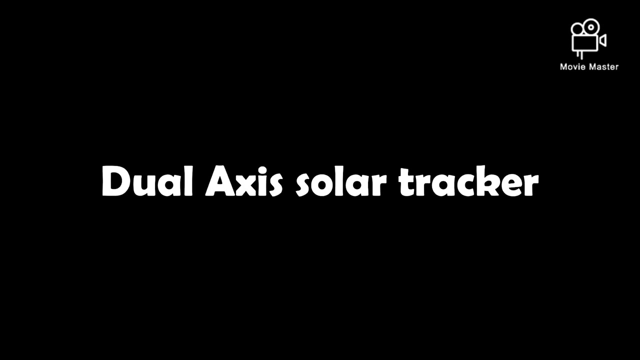 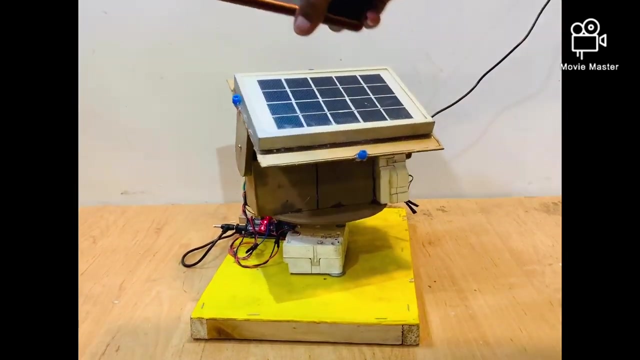 We are heroes tonight. We will fly above the sky. We are heroes tonight. Feel like a dynamite, Ready to explore right up in the sky. I need you to listen, I need you to hear And I'll show Anything. I've been flying from town to town, From London to Taiwan. 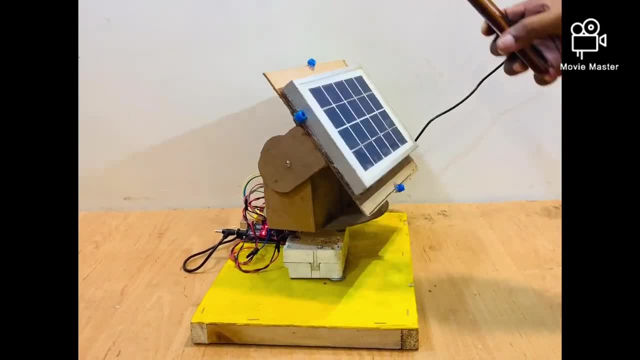 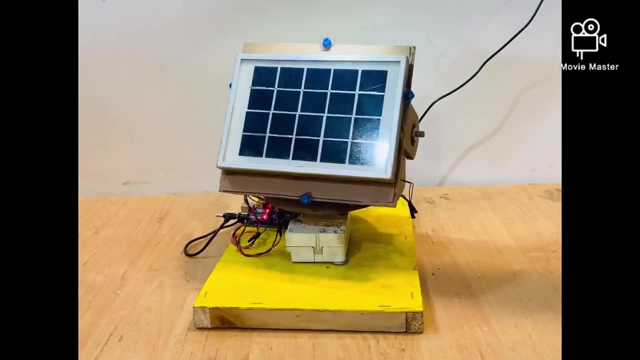 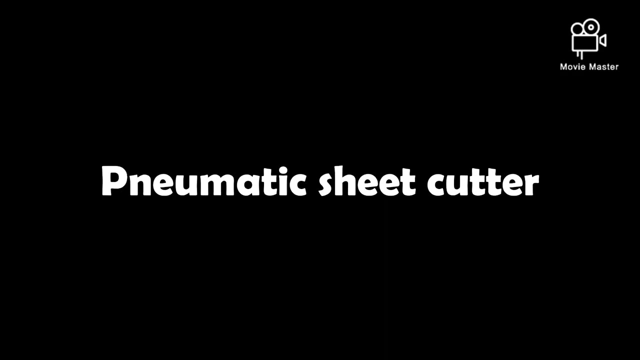 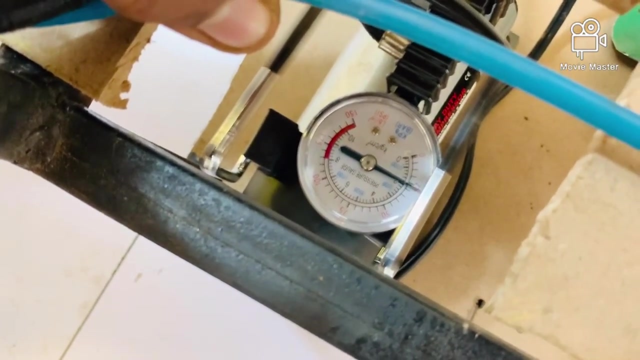 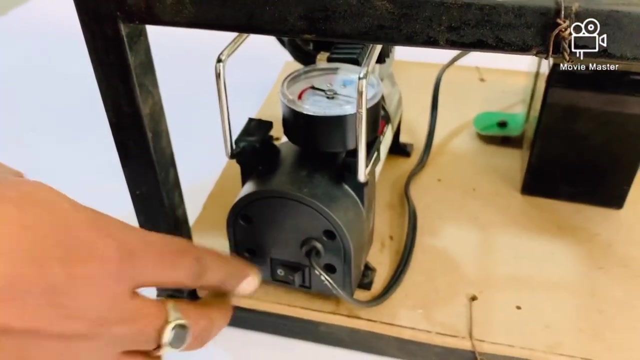 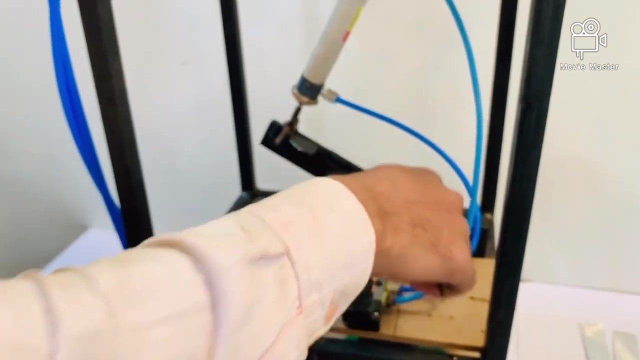 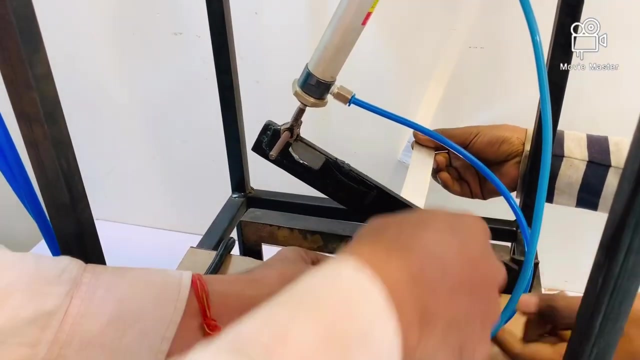 I've been all around the globe Trying to protect your soul. We are heroes tonight. We will fly above the sky. We are heroes tonight. Yeah, Yeah, We are heroes tonight. We will fly above the sky. We are heroes tonight. Yeah, We are heroes tonight. We are heroes tonight. 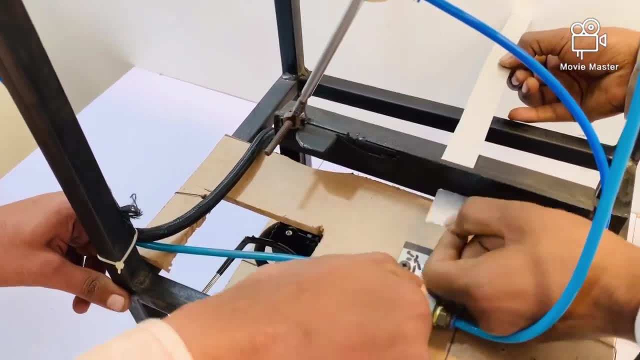 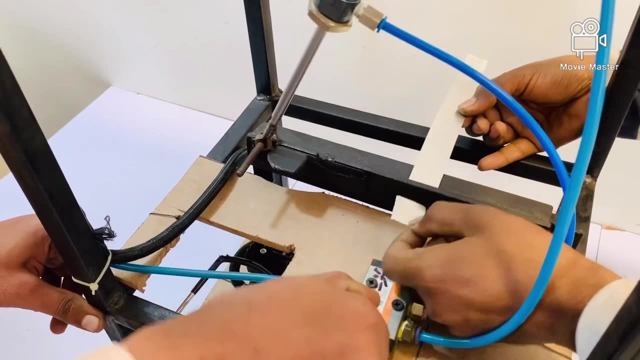 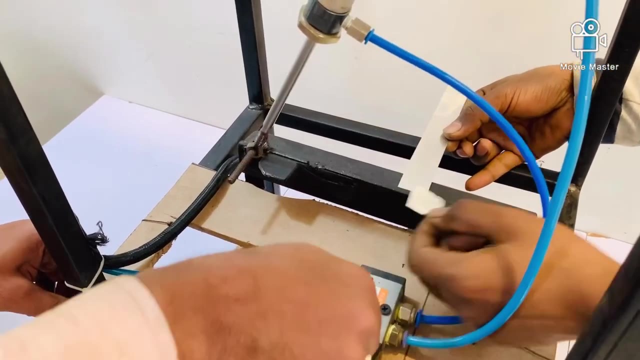 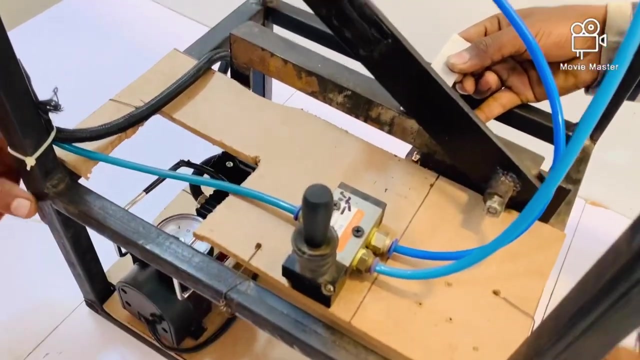